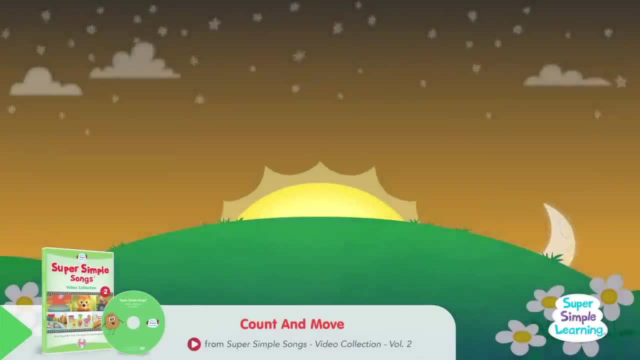 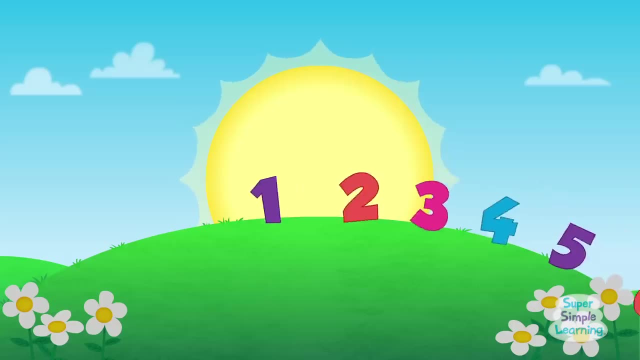 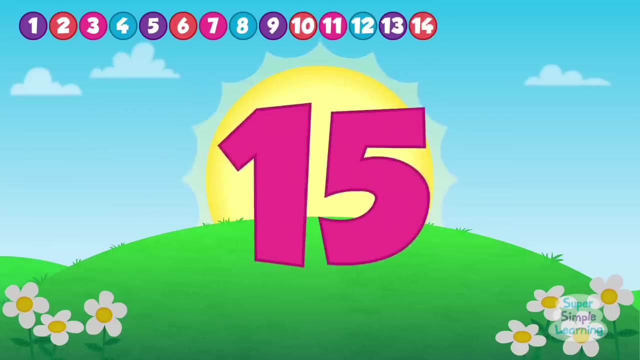 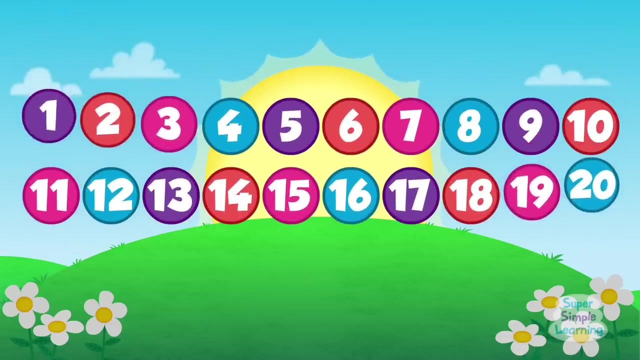 Let's get started with some counting. Can you count to twenty? Here we go. One, Two, Three, Four, Five, Six, Seven, Eight, Nine, Ten, Eleven, Twelve, Thirteen, Fourteen, Fifteen, Sixteen, Seventeen, Eighteen, Nineteen, Twenty. That was fun. 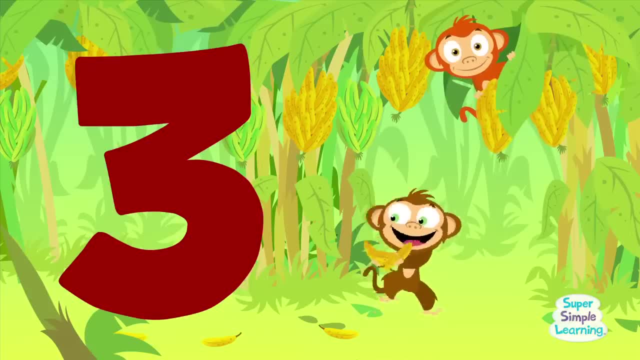 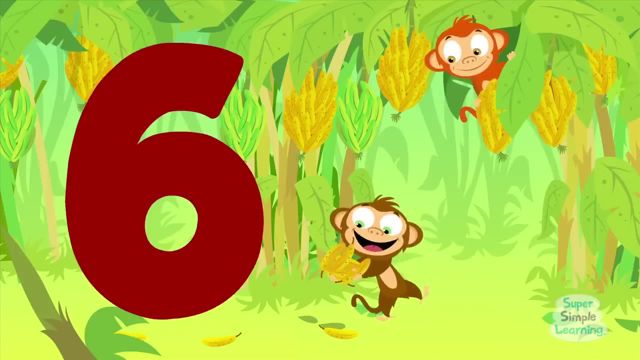 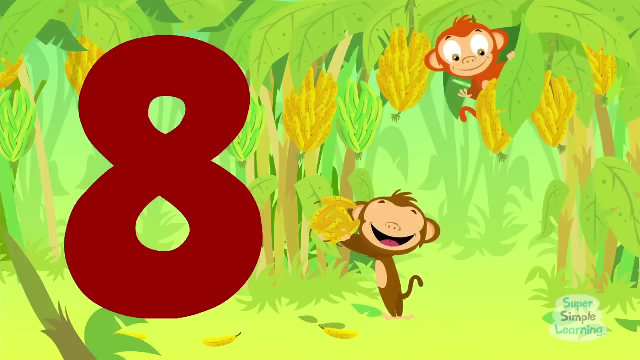 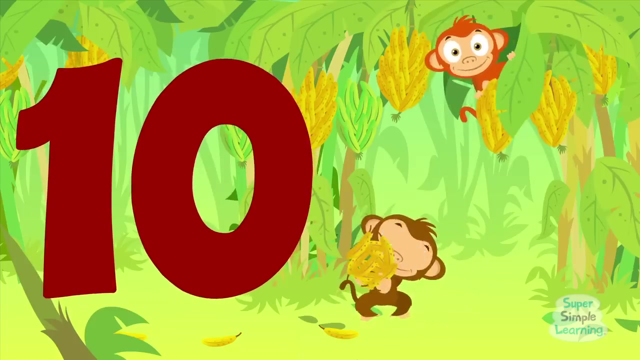 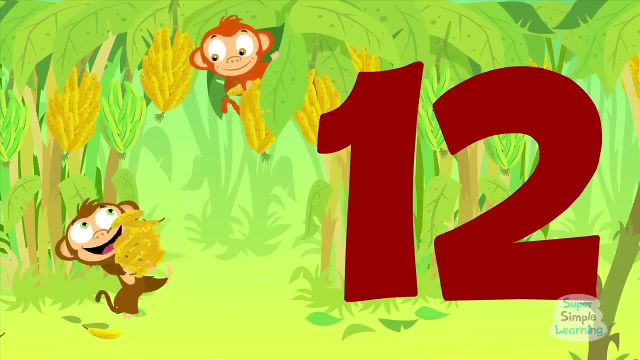 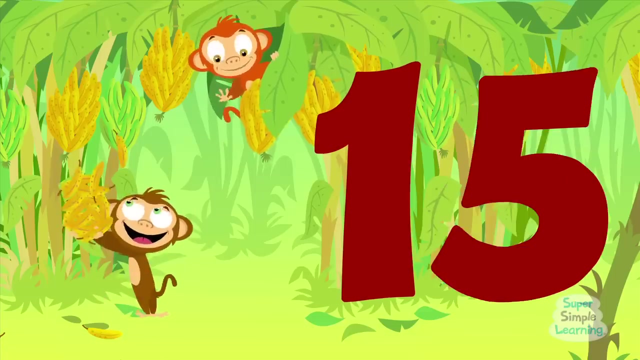 One banana, two bananas, one, two, three, Three bananas for me, Four bananas, five bananas, four, five, six, Six bananas for me Seven, Eight, Nine, Ten, Ten bananas for me Eleven, Twelve, Thirteen, Thirteen bananas for me Fourteen, Fifteen. 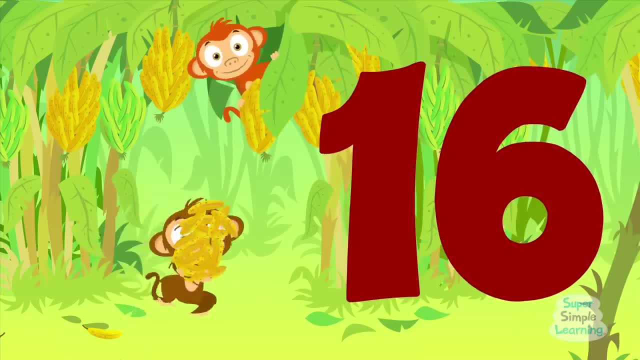 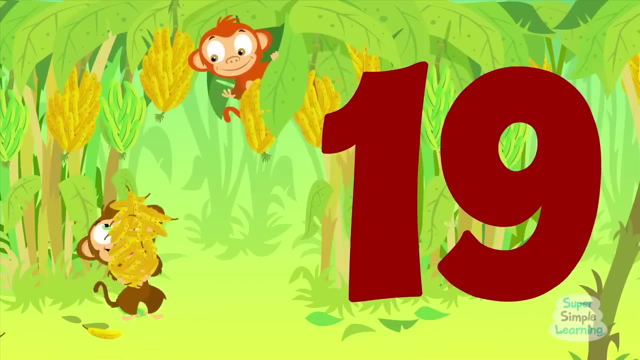 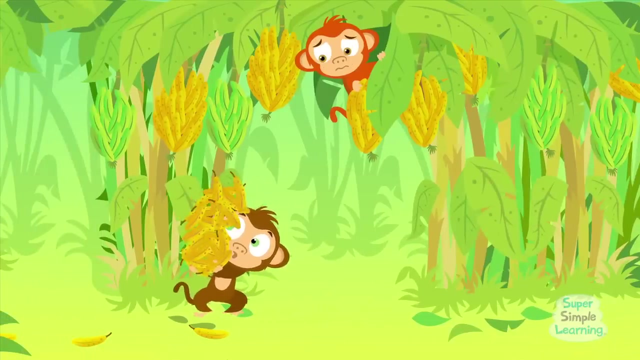 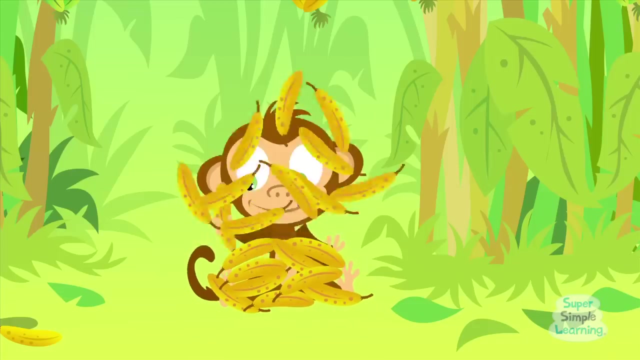 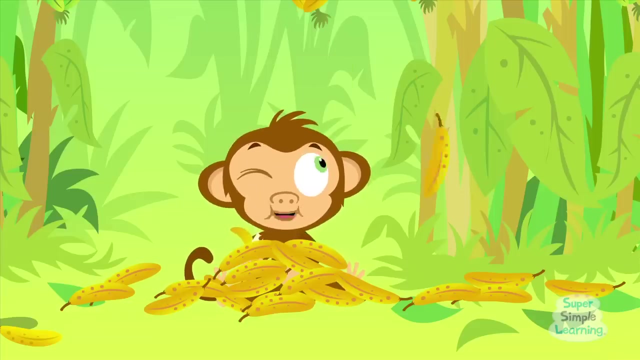 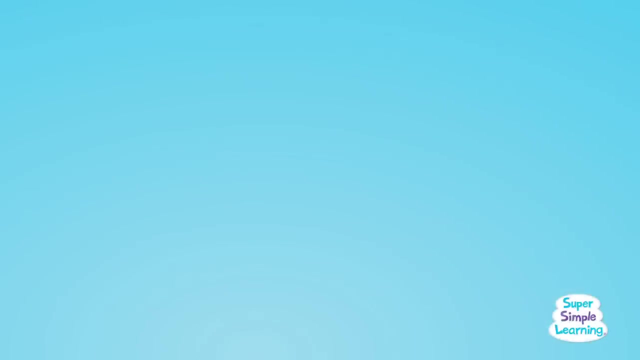 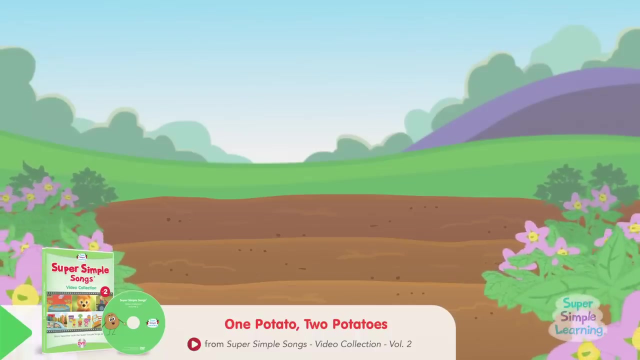 Sixteen, Sixteen bananas for me, 17,, 18,, 19,, 20, 20 bananas for me. Bananas to the left, Bananas to the right. Bananas- turn around Bananas. sit down Now, peel your bananas and take a bite. One potato, two potatoes, three potatoes, four. 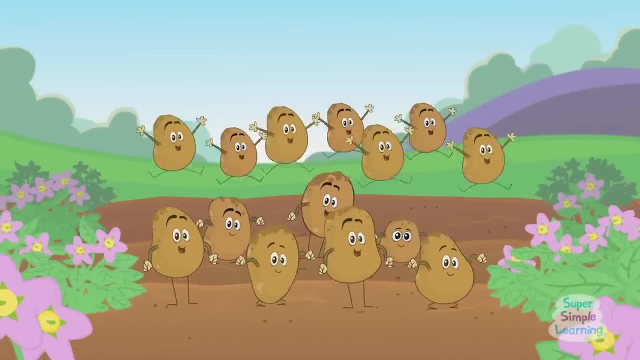 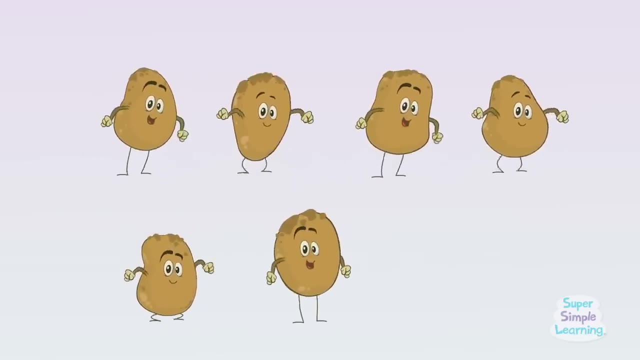 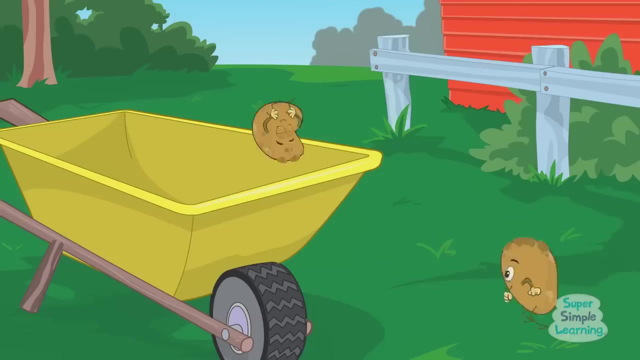 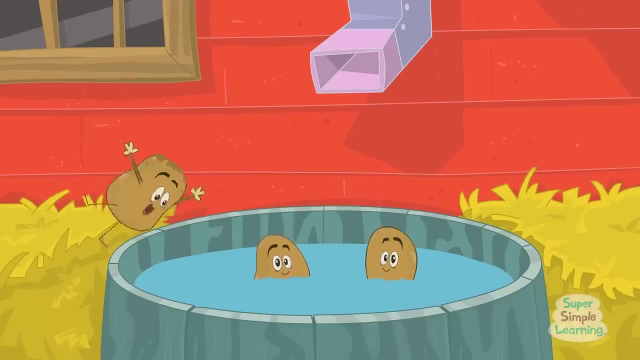 Five potatoes, six potatoes, seven potatoes more One potato, two potatoes, three potatoes, four, Five potatoes, six potatoes, seven potatoes more One potato, two potatoes, three potatoes, four, Five potatoes, six potatoes, seven potatoes more One potato, two potatoes, three potatoes, four. 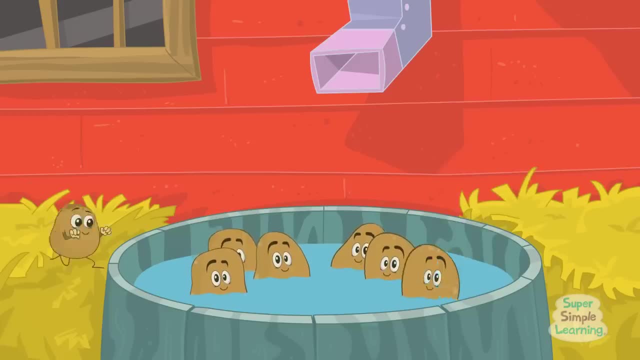 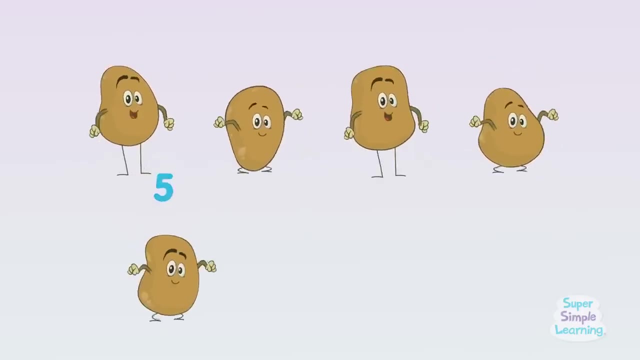 Five potatoes, six potatoes, seven potatoes more. 5 Potatoes, 6 Potatoes, 7 Potatoes more. 1 Potato, 2 Potatoes, 3 Potatoes, 4, 5 Potatoes, 6 Potatoes, 7 Potatoes more. 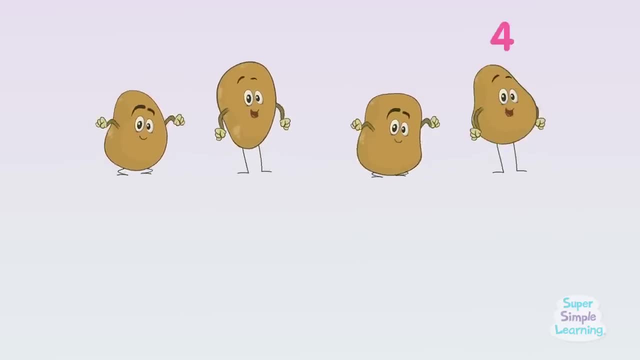 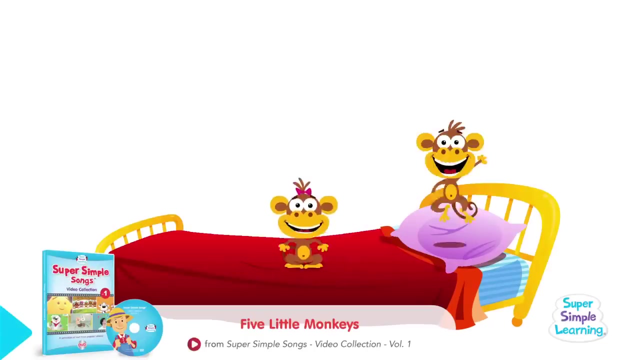 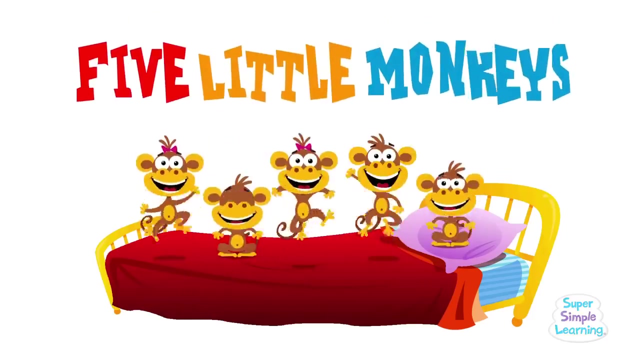 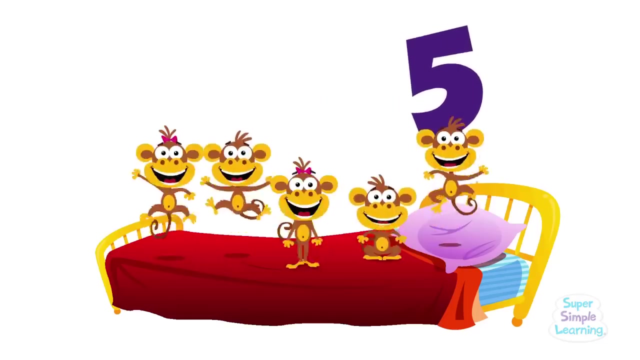 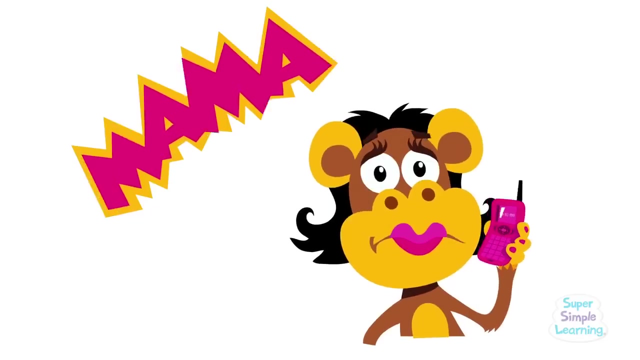 1 Potato, 2 Potatoes, 3 Potatoes, 4, 5 Potatoes, 6 Potatoes, 7 Potatoes, more, 5 Little Monkeys Jumping On The Bed. One fell off and bumped his head. Mama called the doctor and the doctor said: 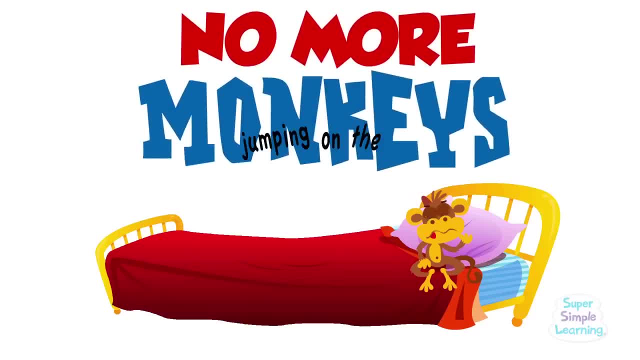 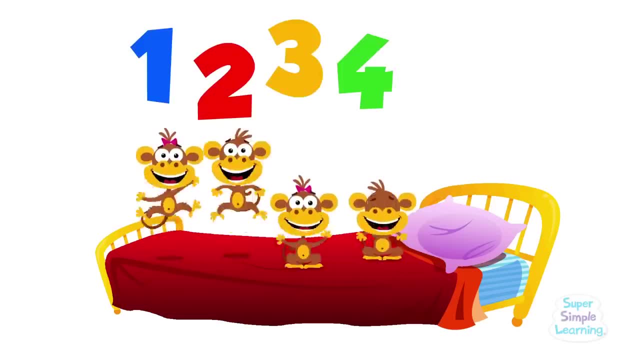 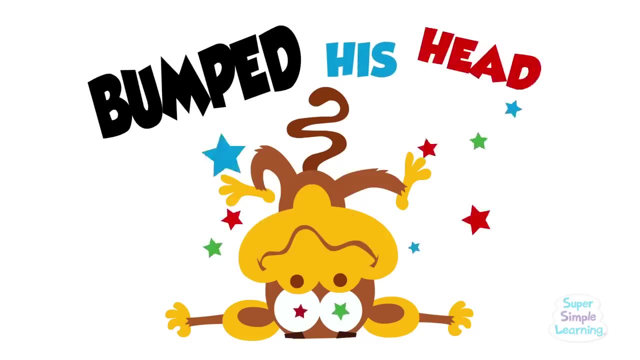 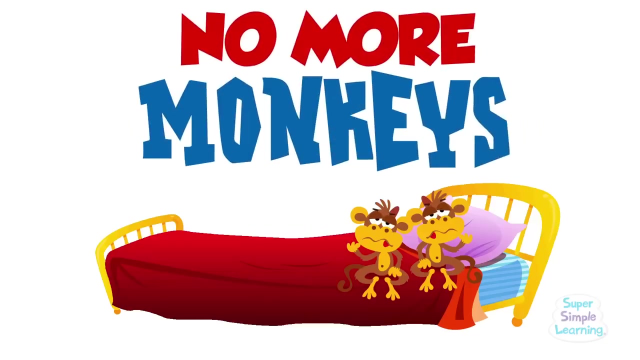 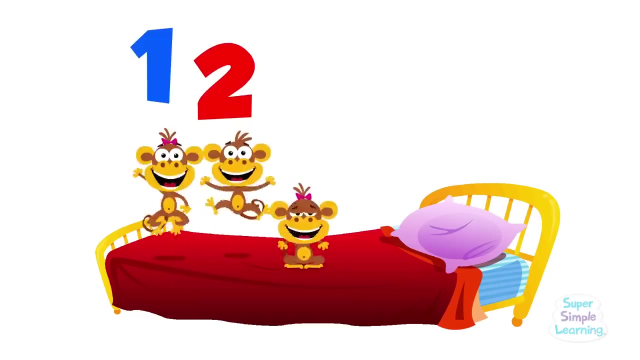 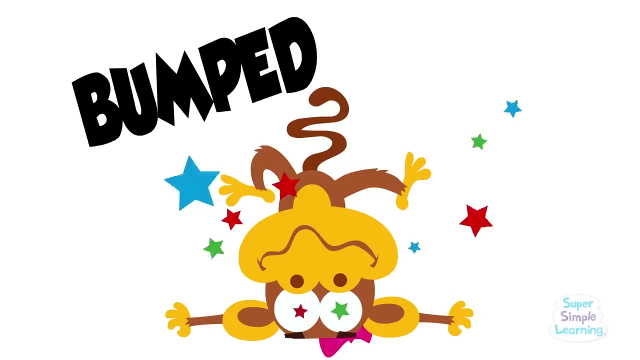 No more monkeys jumping on the bed. 4 Little Monkeys Jumping On The Bed. One fell off and bumped his head. Mama called the doctor and the doctor said: No more monkeys jumping on the bed. 3 Little Monkeys Jumping On The Bed. One fell off and bumped her head. 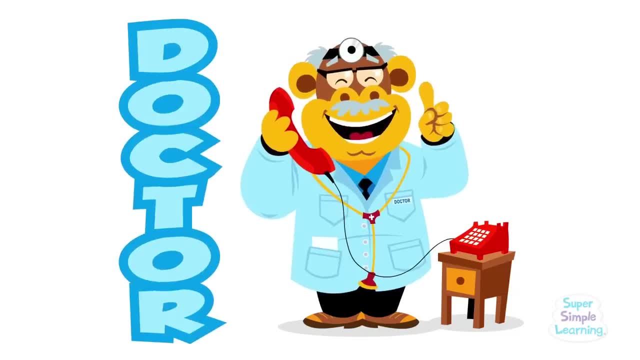 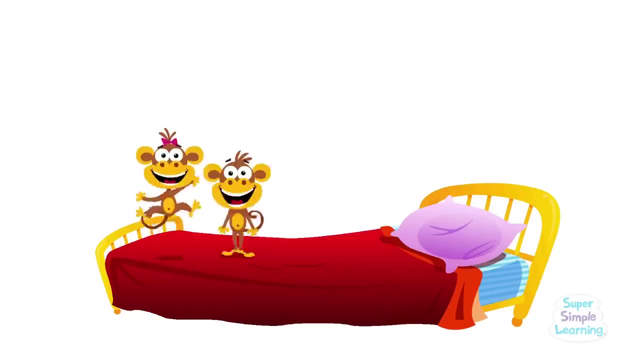 Mama called the doctor and the doctor said: No more monkeys jumping on the bed. 2 Little Monkeys Jumping On The Bed. 1 Little Monkeys Jumping On The Bed. 1 Little Monkeys Jumping On The Bed. 1 Little Monkeys Jumping On The Bed. 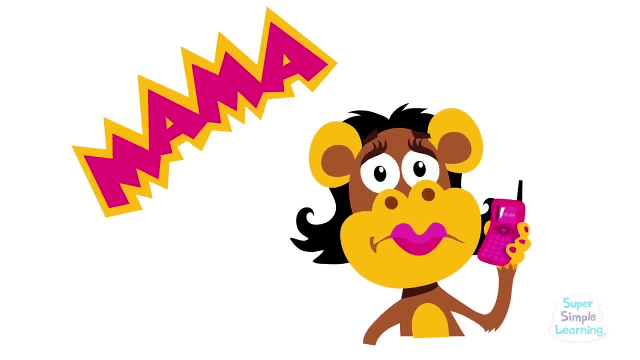 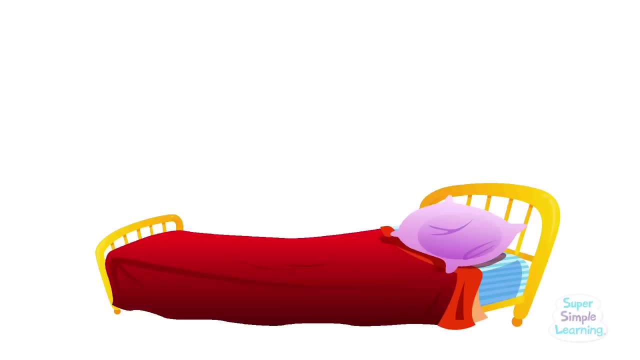 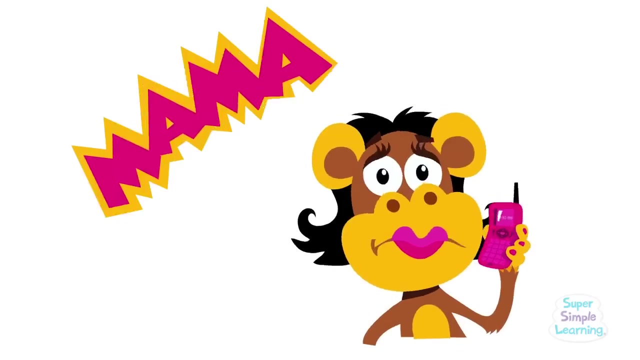 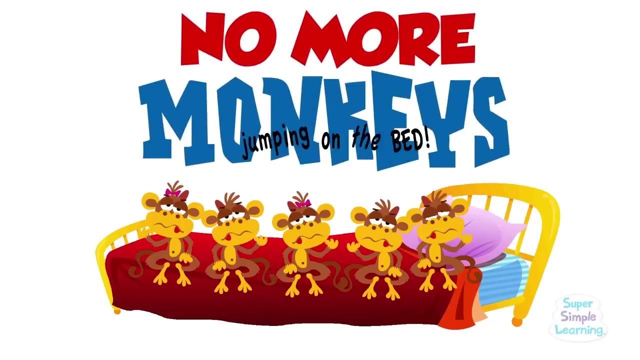 Mama called the doctor and the doctor said: No more monkeys jumping on the bed. 1- Little Monkeys Jumping On The Bed. She fell off and bumped her head. Mama called the doctor and the doctor said: No more monkeys jumping on the bed. 2- Little Monkeys Jumping On The Bed. 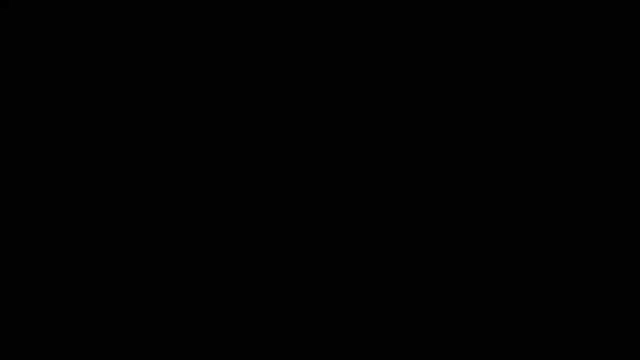 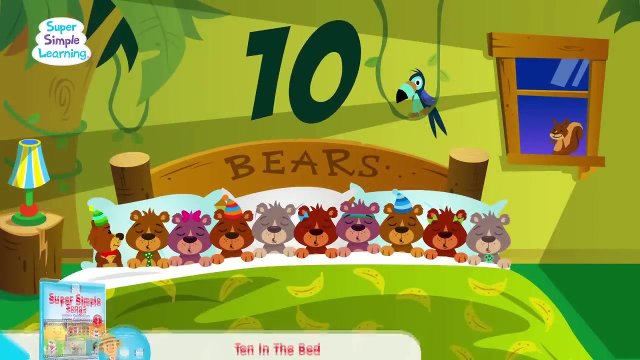 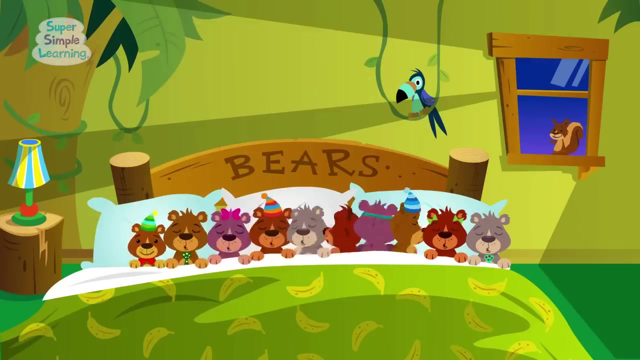 Mama called the doctor and the doctor said: No more monkeys jumping on the bed, Here we go. There were ten in the bed And the little one said: Roll over, roll over. So they all rolled over And one fell out Nine. There were nine in the bed. 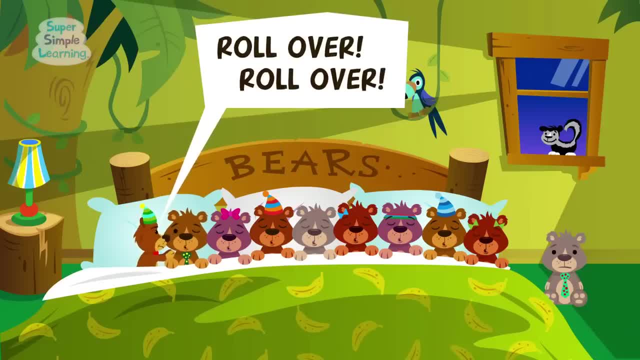 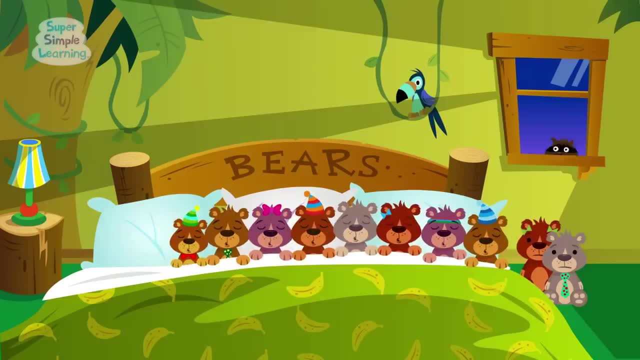 And the little one said: Rolled over, rolled over. So they all rolled over and one fell out Eight. There were eight in the bed and the little one said: Rolled over, rolled over. So they all rolled over and one fell out Seven. There were seven in the bed and the little one said: 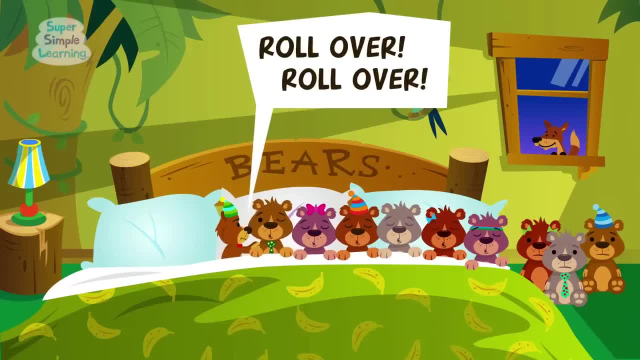 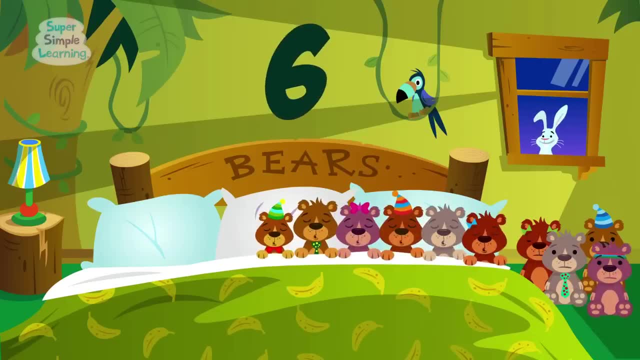 Rolled over, rolled over. So they all rolled over and one fell out Six. There were six in the bed and the little one said: Rolled over, rolled over. So they all rolled over and one fell out Five. There were five in the bed and the little one said: 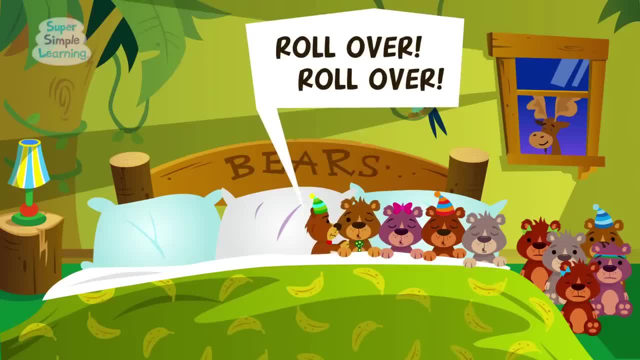 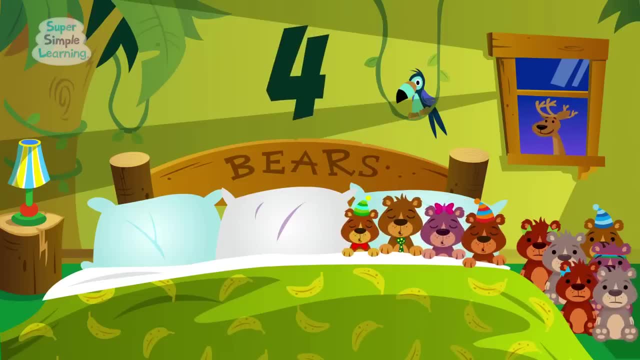 Rolled over. So they all rolled over and one fell out Four. There were four in the bed and the little one said: Roll over, roll over. So they all rolled over and one fell out Three. There were three in the bed and the little one said: Roll over, roll over. 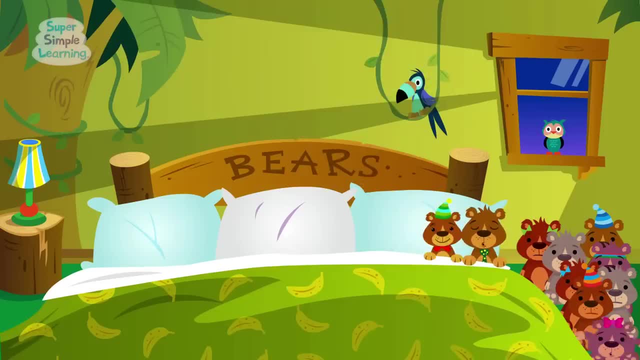 So they all rolled over and one fell out Two. There were two in the bed and the little one said: Roll over, roll over. So they both rolled over and one fell out One. There was one in the bed and the little one said: I'm lonely, I'm lonely. 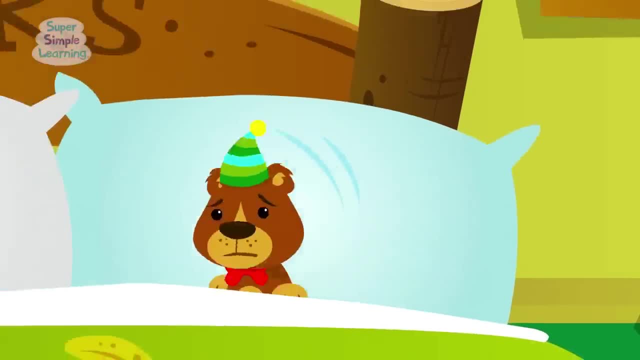 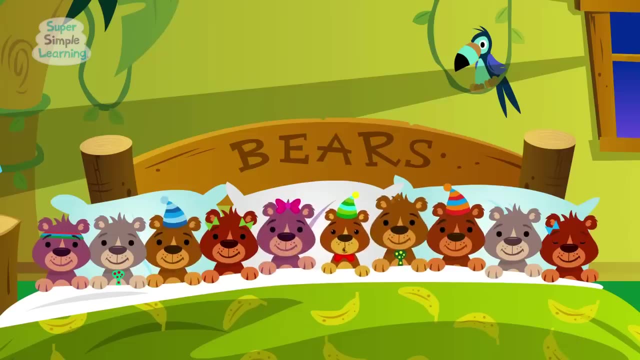 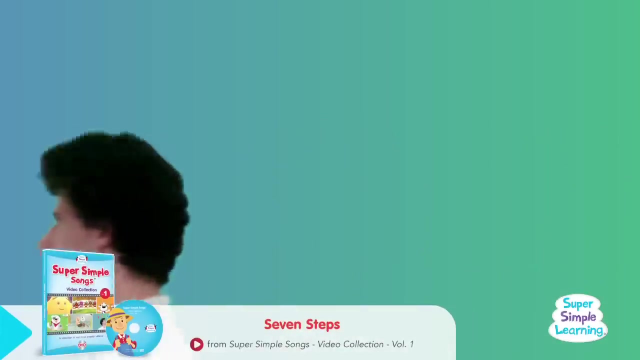 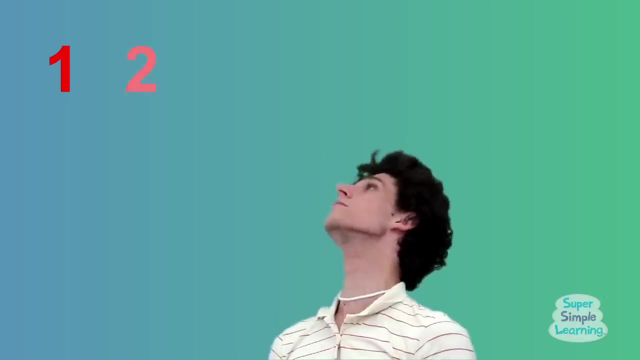 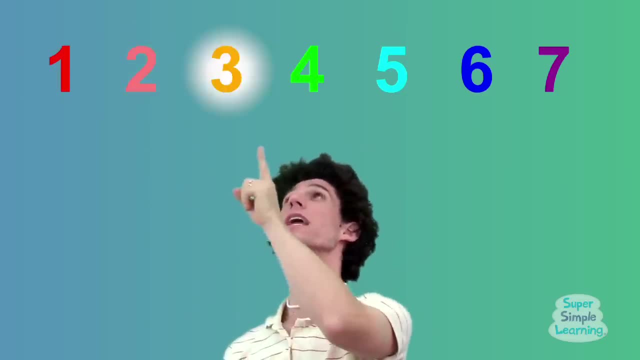 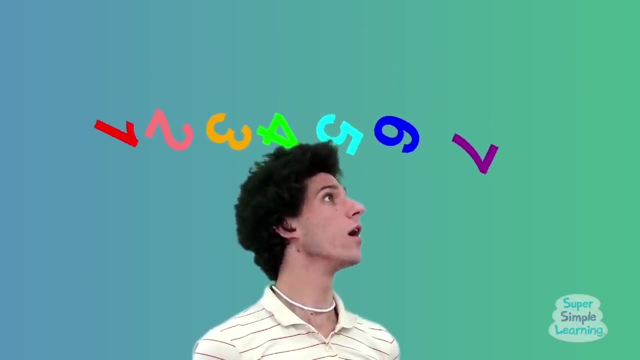 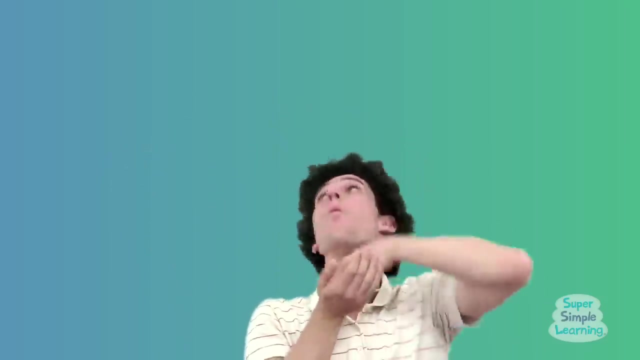 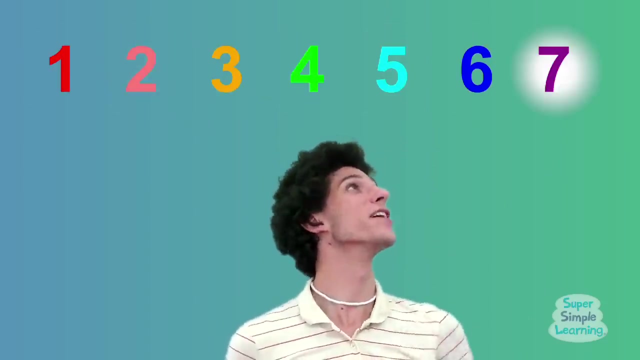 One, two, three, four, five, six, seven. One, two, three, four, five, six, seven. One, two, three, four, five, six seven. One, two, three. One, two, three, four, five, six, seven. 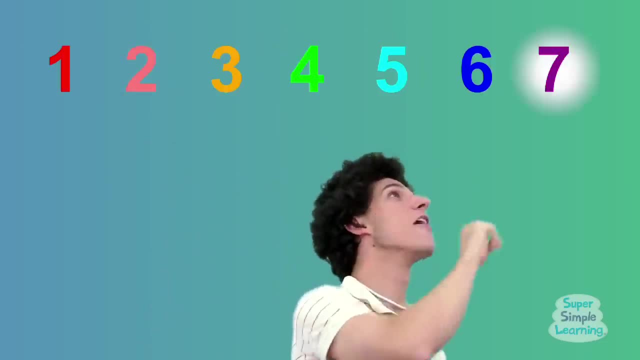 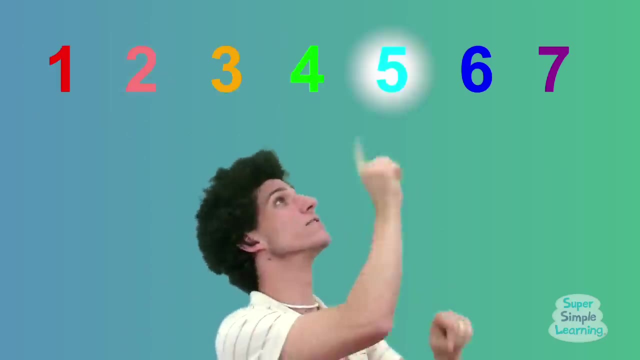 1, 2,, 3,, 4,, 5,, 6, 7, 1, 2, 3, 1, 2, 3, 1, 2,, 3,, 4,, 5,, 6, 7. 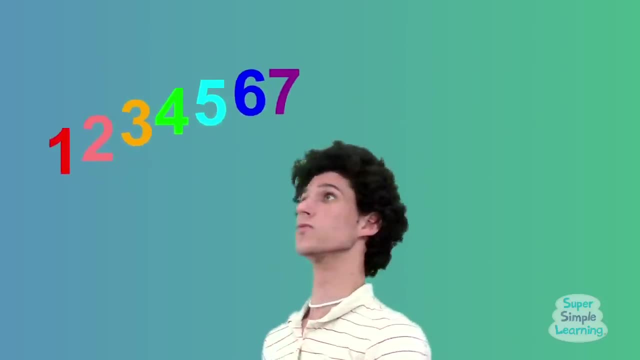 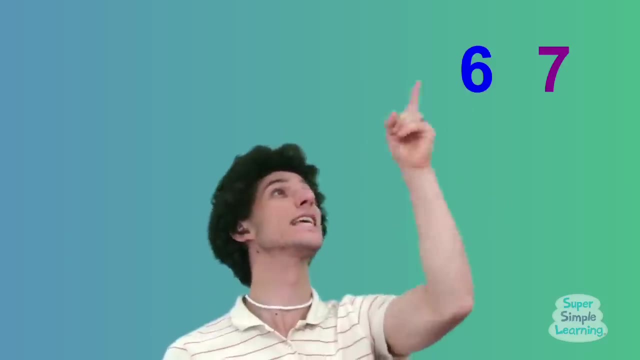 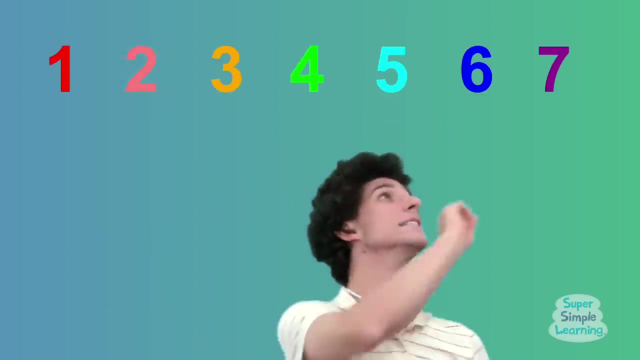 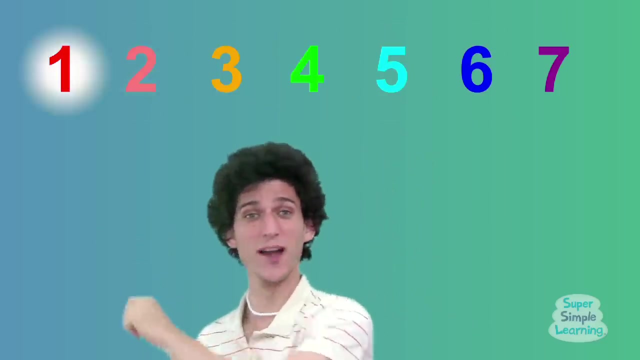 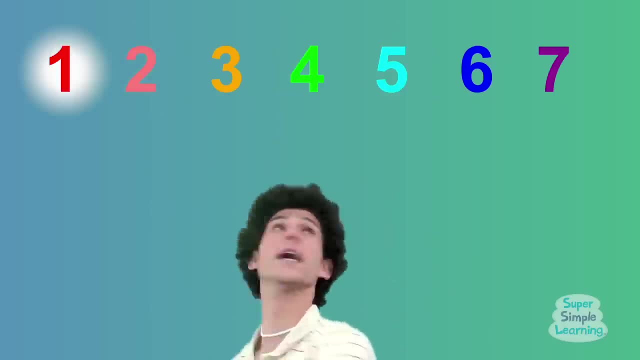 7, 6, 5,, 4,, 3, 2, 1, 7, 6, 5,, 4,, 3, 2, 1, 5, 4, 3, 2, 1. 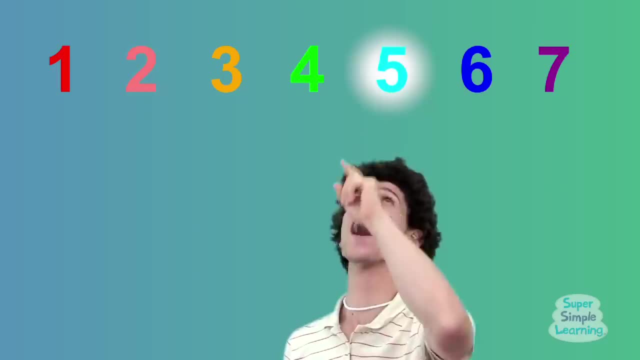 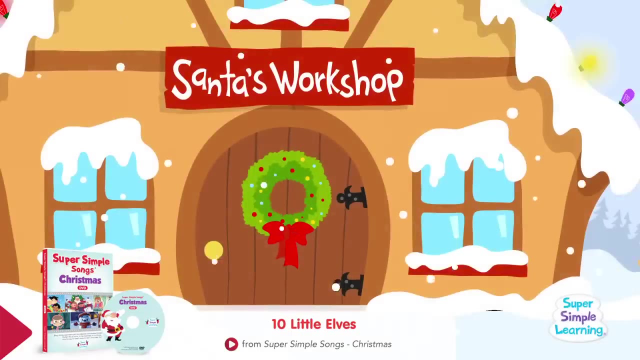 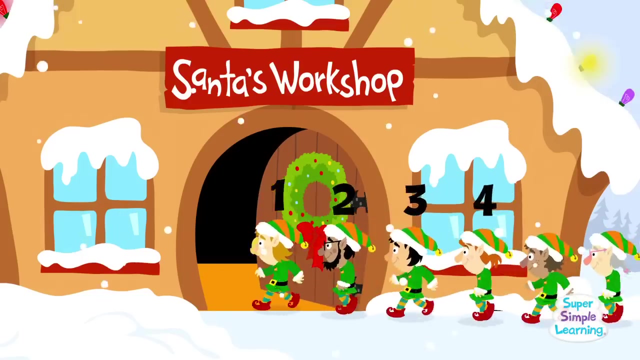 7, 6, 5, 7, 6, 5, 7, 6, 5, 4, 3, 2, 1. 1 little 2. little 3 little elves. 4 little 5. little 6 little elves. 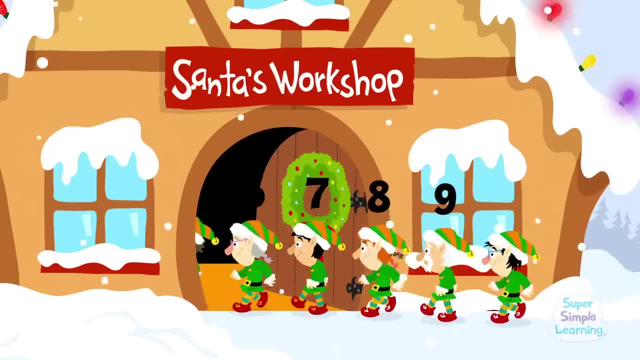 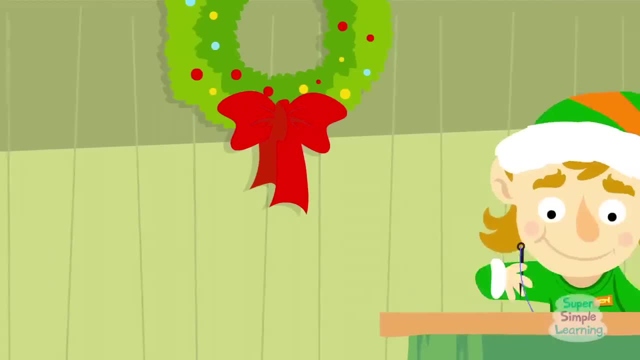 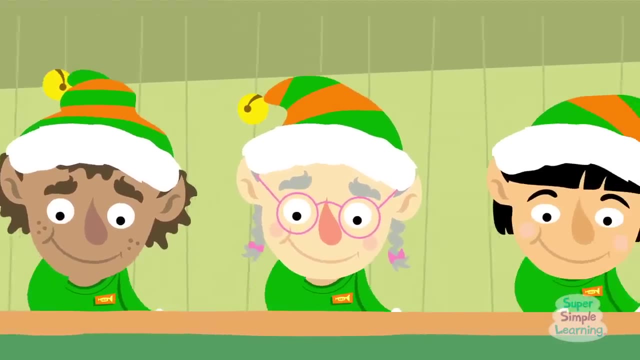 7 little, 8 little, 9 little elves. 10 little elves are making toys: 1 little, 2 little, 3 little elves. 4 little, 5 little, 6 little elves. 7 little, 8 little, 9 little elves. 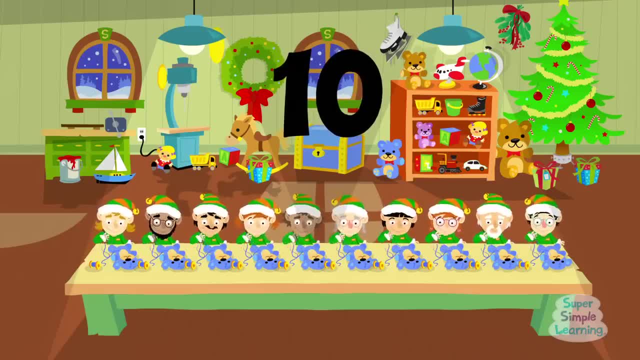 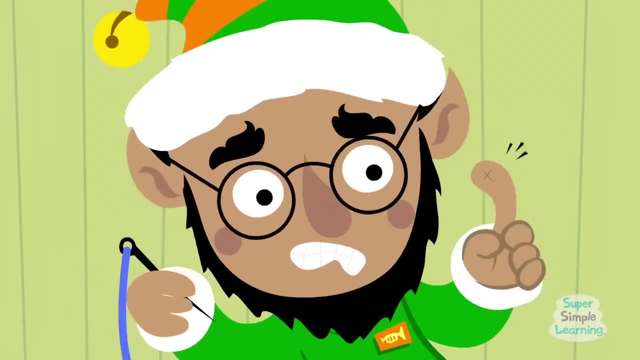 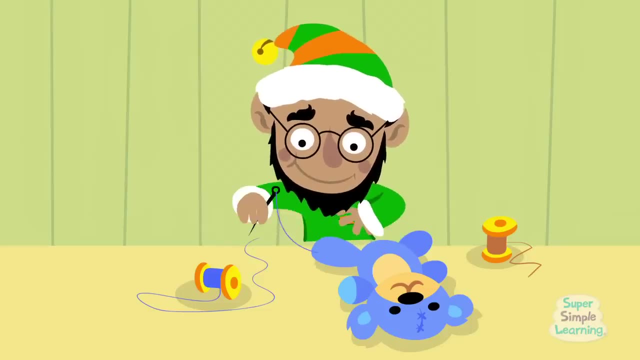 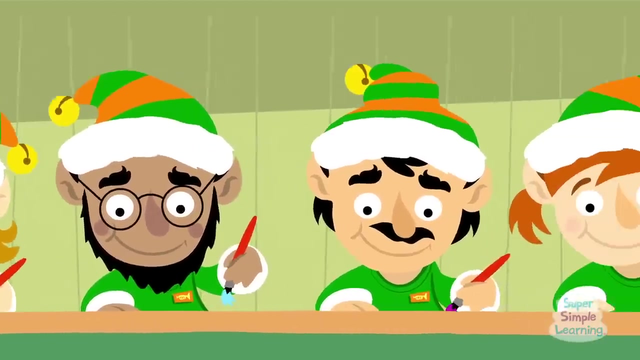 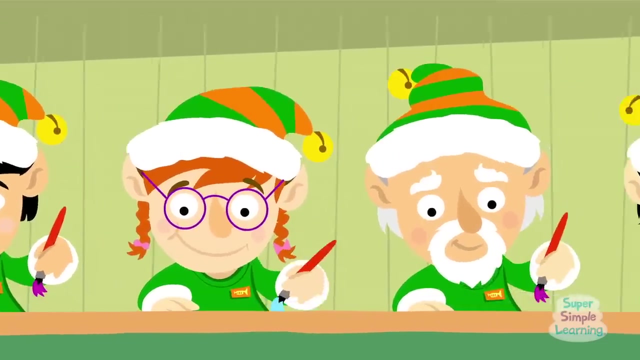 10 little elves are sewing. Ouch, Hurry up 1 little, 2 little, 3 little elves, 4 little, 5 little, 6 little elves, 7 little, 8 little, 9 little elves, 10 little elves are painting. 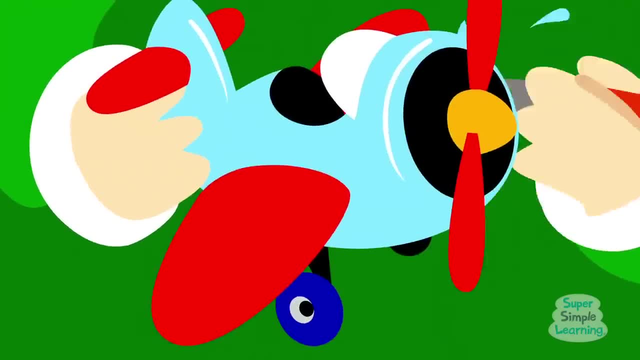 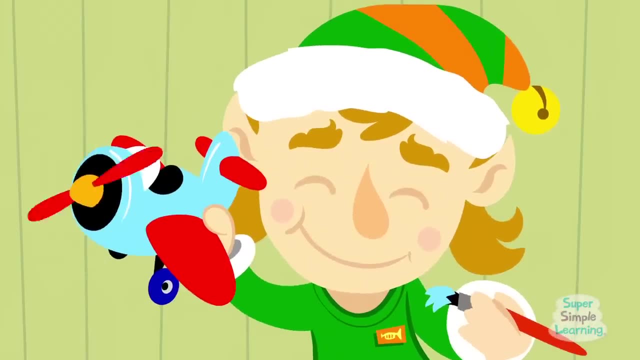 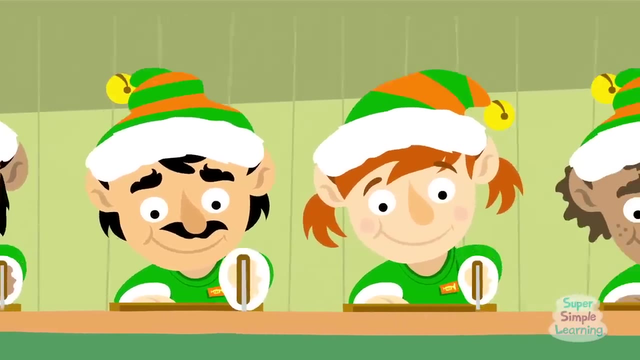 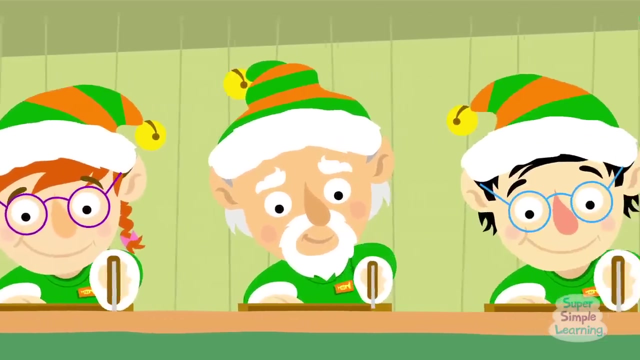 We need more colors over here. Hey, that's pretty, Santa's gonna like that. one. 1 little, 2 little, 3 little elves. 4 little, 5 little, 6 little elves. 7 little, 8 little, 9 little elves. 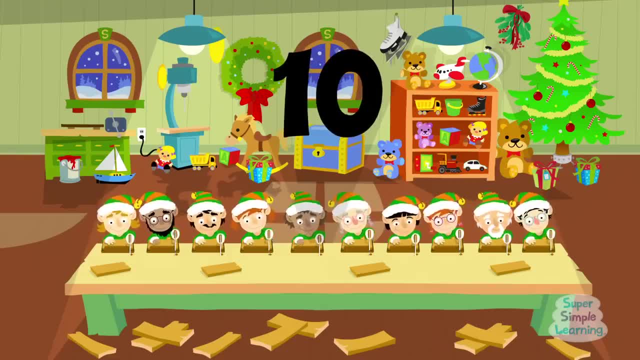 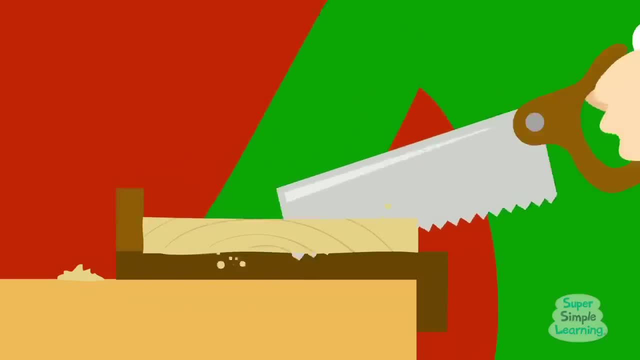 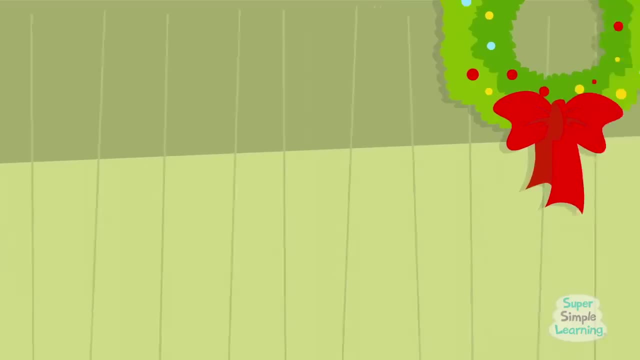 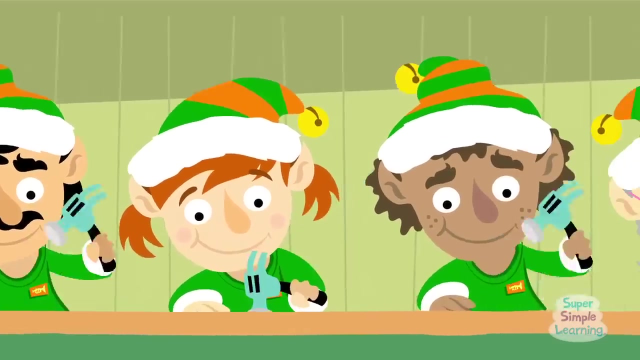 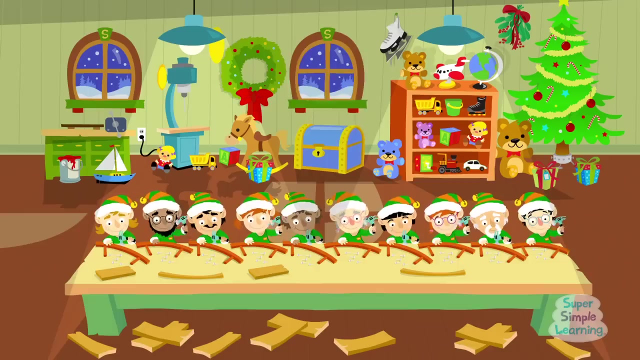 10 little elves are sawing. Be careful with that thing. That looks great. Anybody seen the safety goggles? 1 little- 2 little, 3 little elves. 4 little- 5 little, 6 little elves. 7 little- 8 little, 9 little elves. 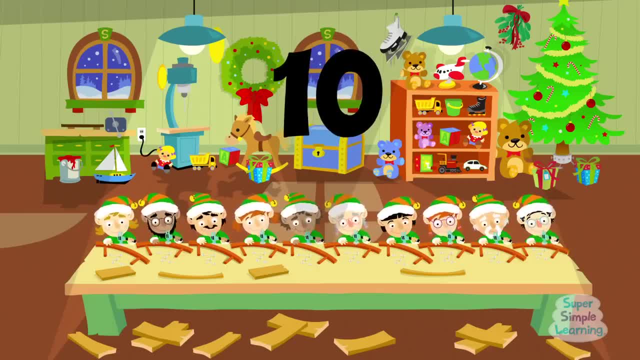 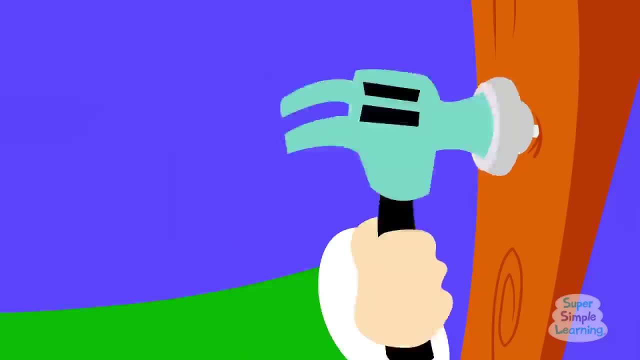 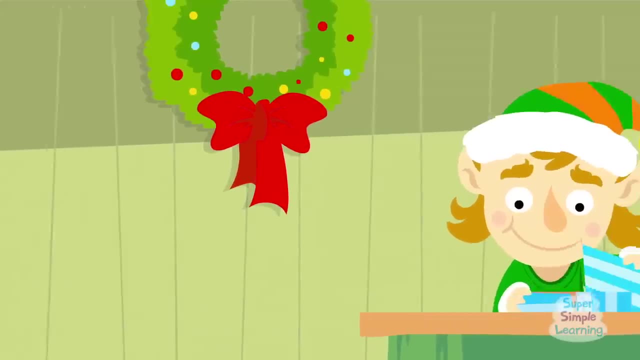 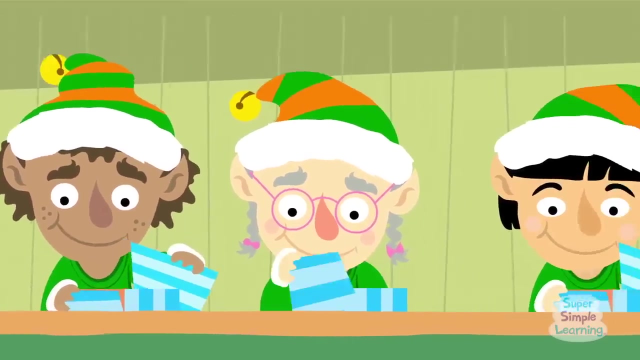 10 little elves are hammering. I need some nails over here. That looks great. 1 little, 2 little, 3 little elves. 4 little, 5 little, 6 little elves. 7 little, 8 little, 9 little elves. 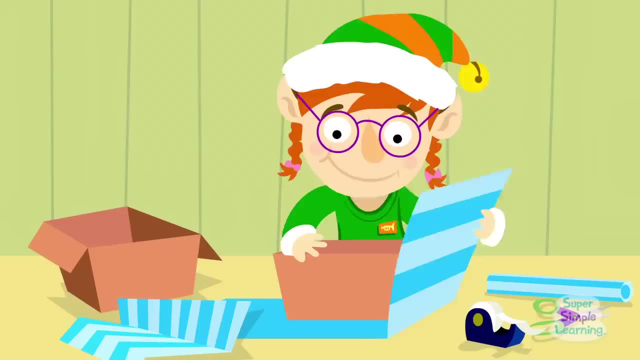 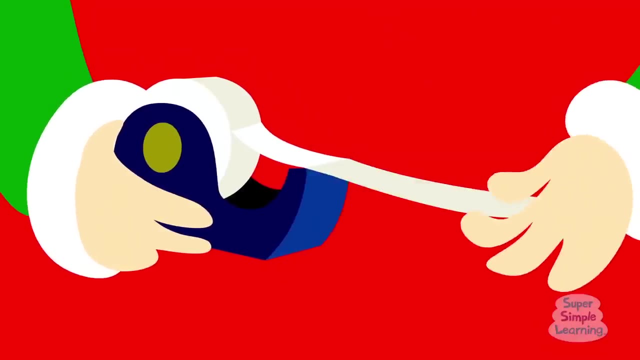 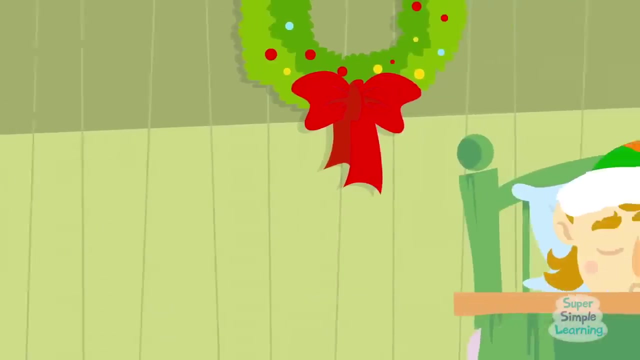 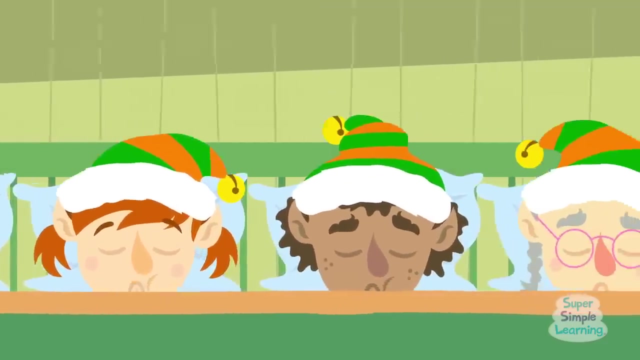 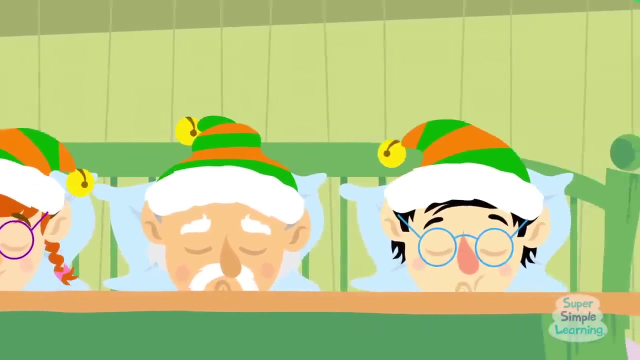 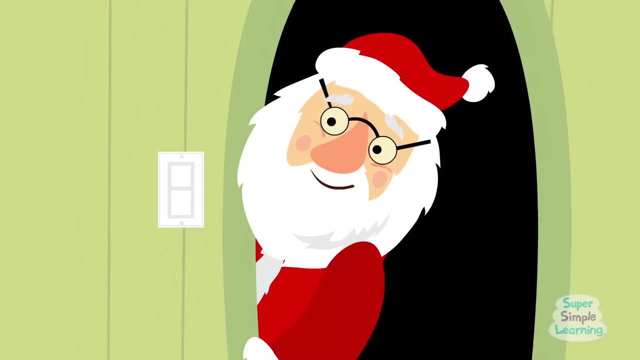 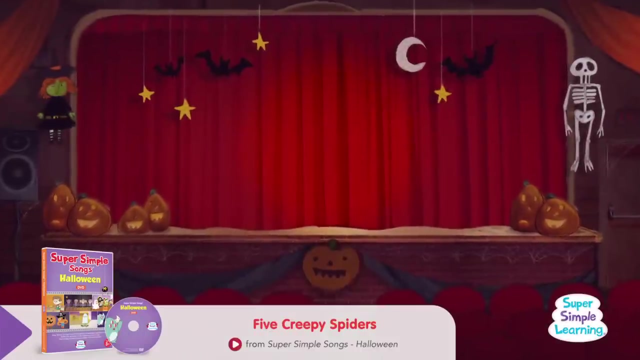 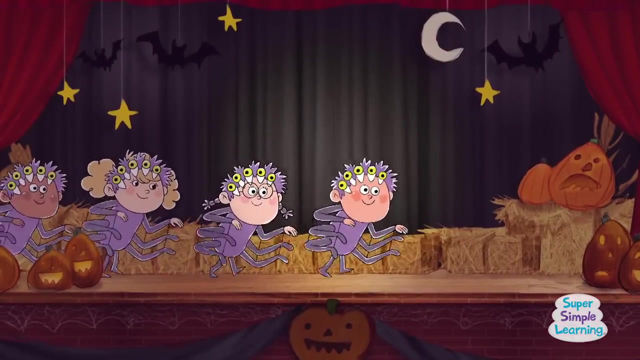 10 little elves are wrapping Racking. Have you seen the tape? Pass the scissors. One little, two little three little elves. four little five little six little elves. seven little, eight little nine little elves. ten little elves are sleeping. Five creepy spiders. five creepy spiders. see how they crawl. 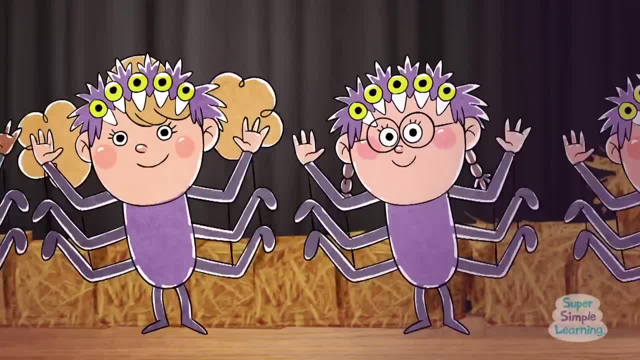 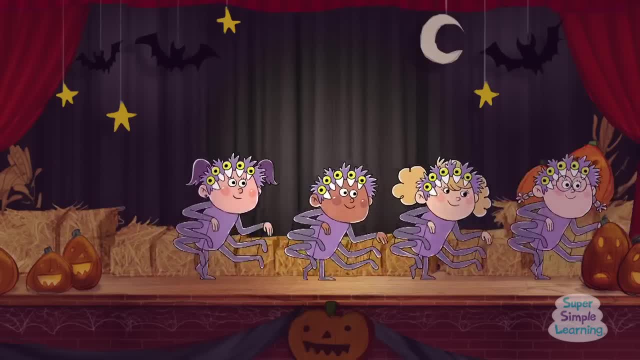 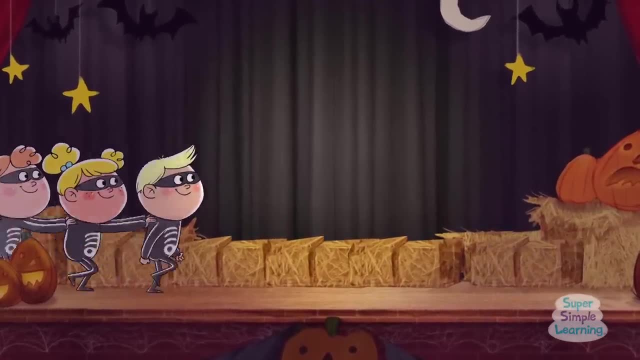 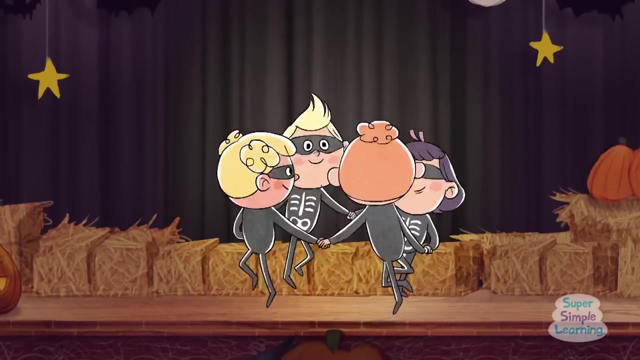 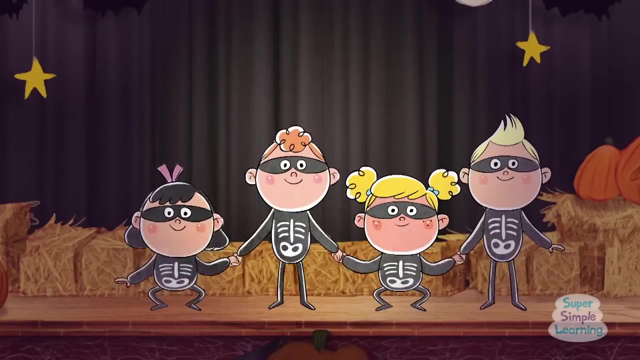 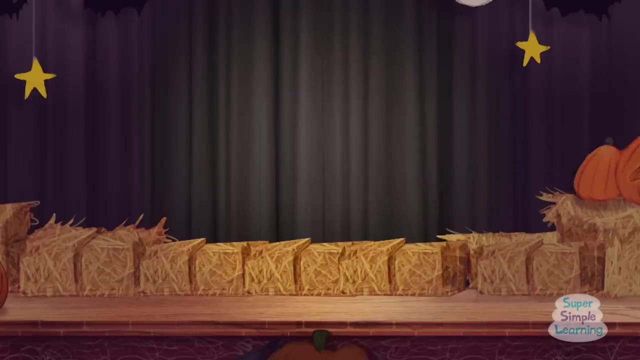 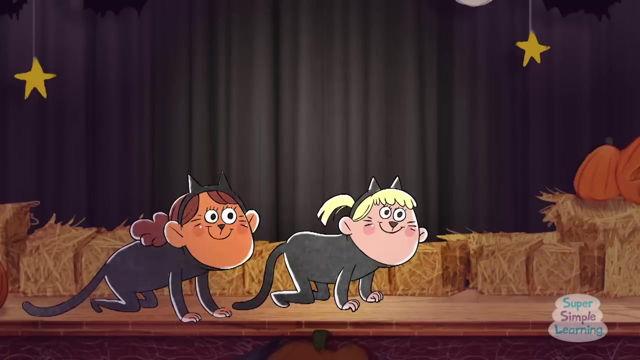 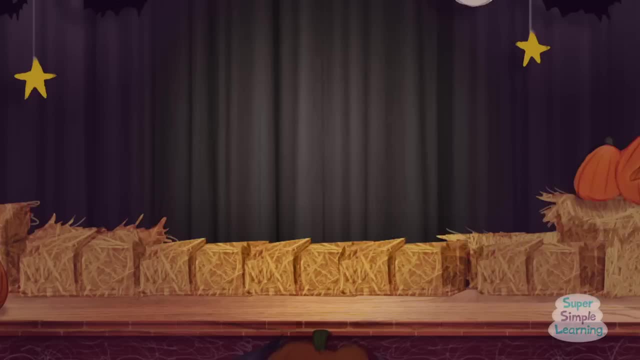 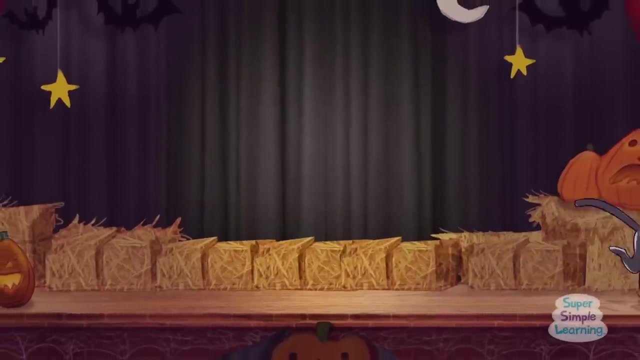 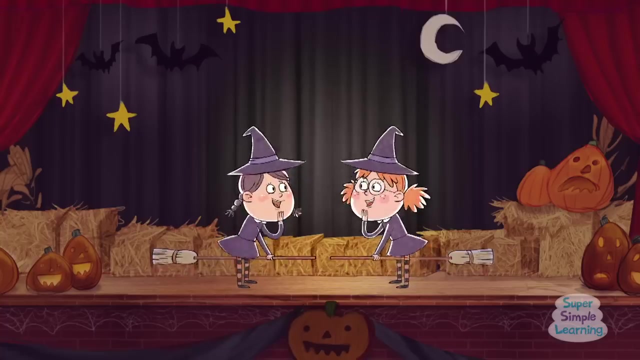 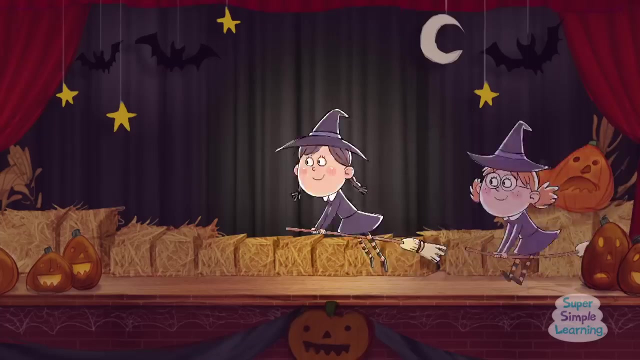 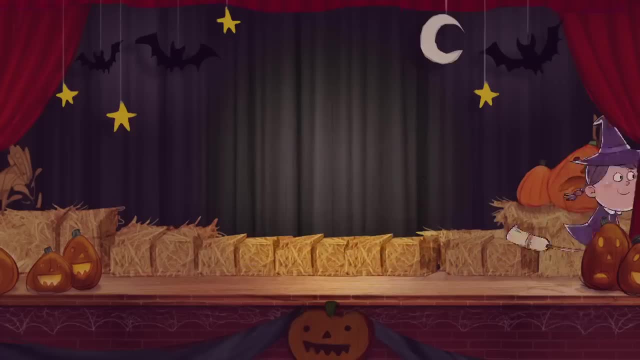 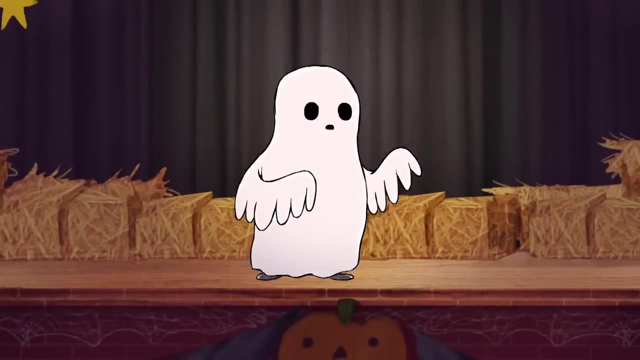 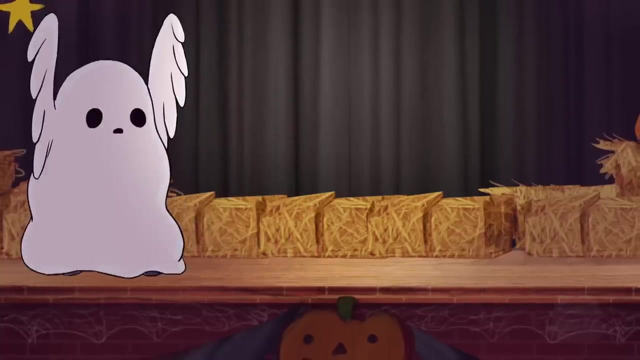 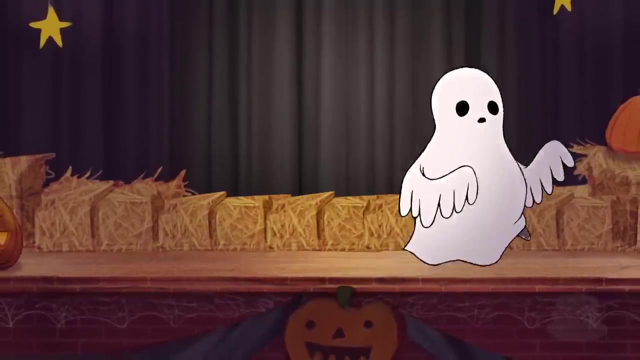 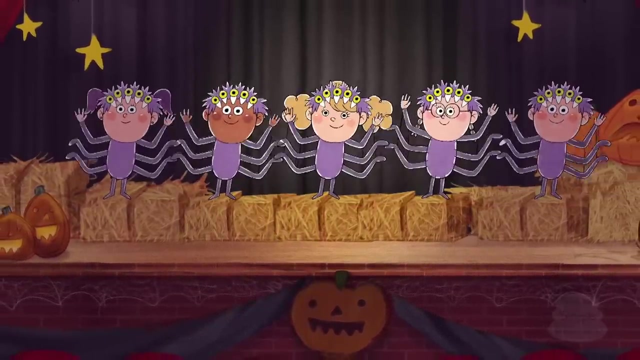 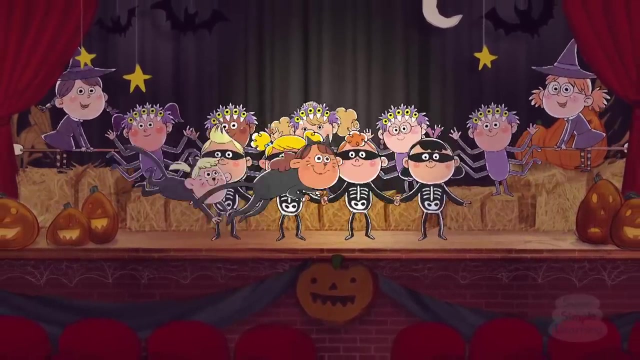 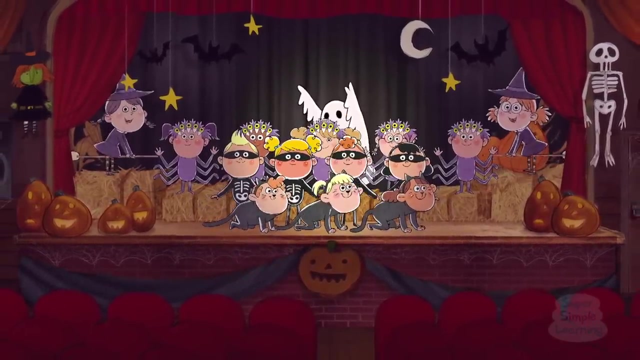 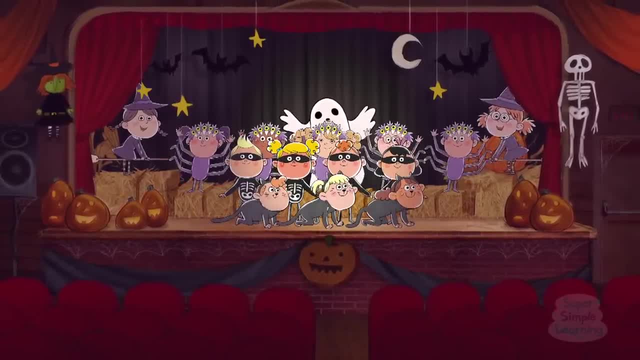 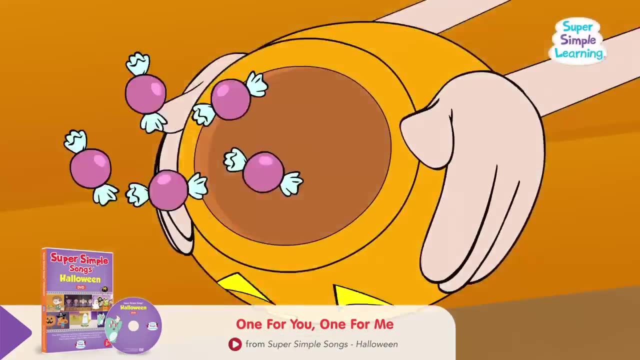 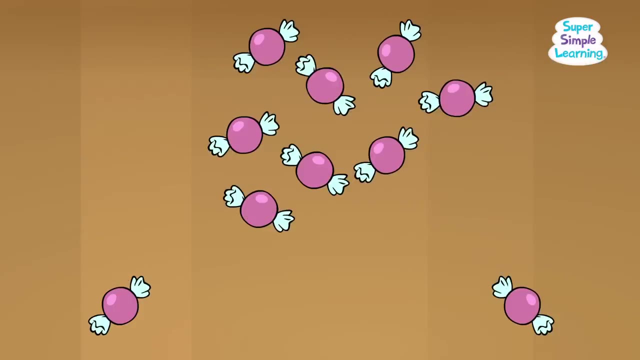 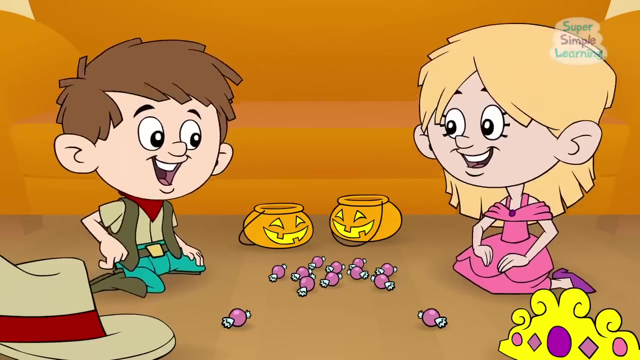 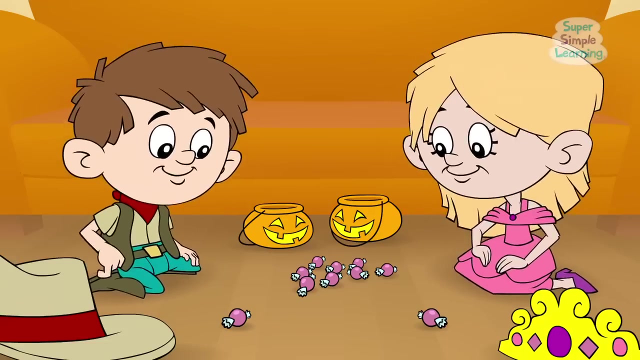 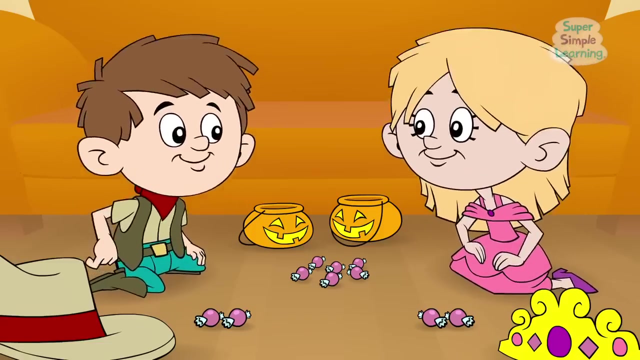 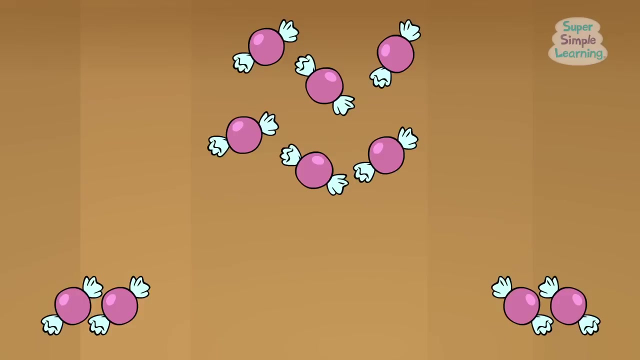 Happy Halloween. Happy Halloween- One for you, one for me. Let's share all of our candy. Happy happy Halloween- One for you, one for me, Two for you, two for me. Let's share all of our candy. Happy happy Halloween. Two for you, two for me. 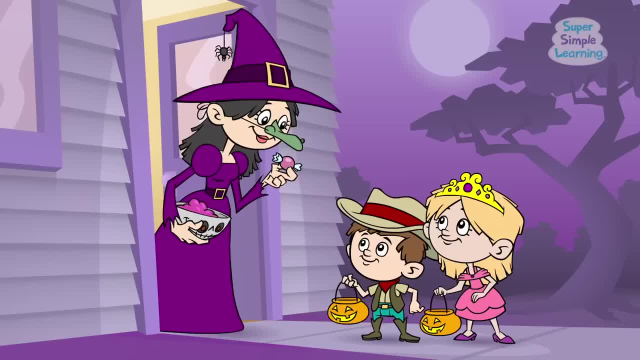 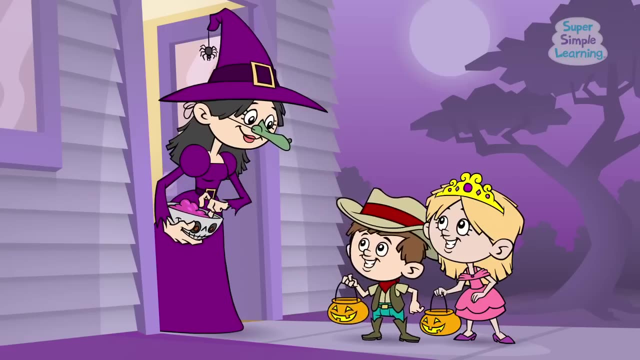 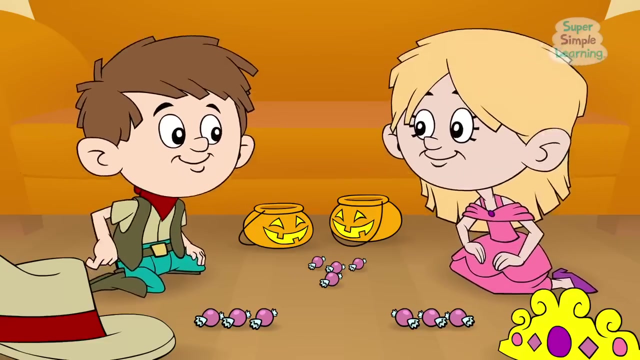 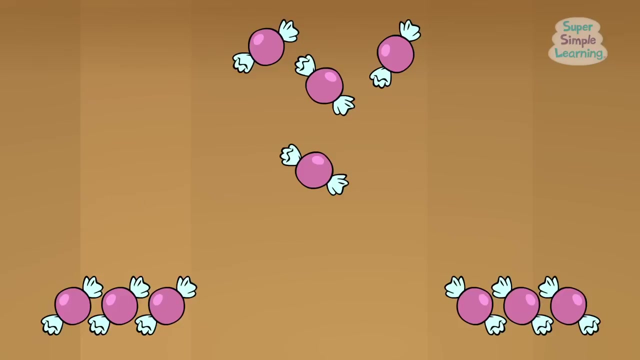 Here you are, Thank you very much. Here you are, Thank you very much. Three for you, three for me. Let's share all of our candy. Happy, happy Halloween. Three for you, three for me, Four for you, four for me. Let's share all of our candy.